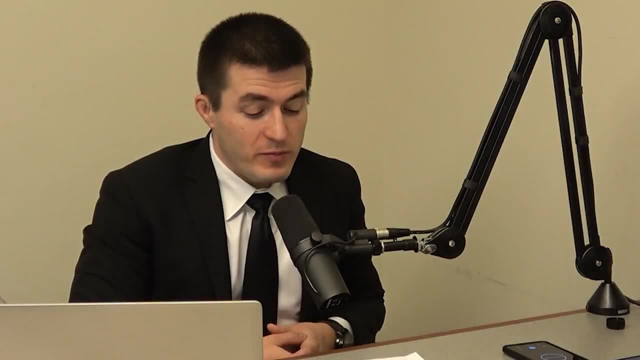 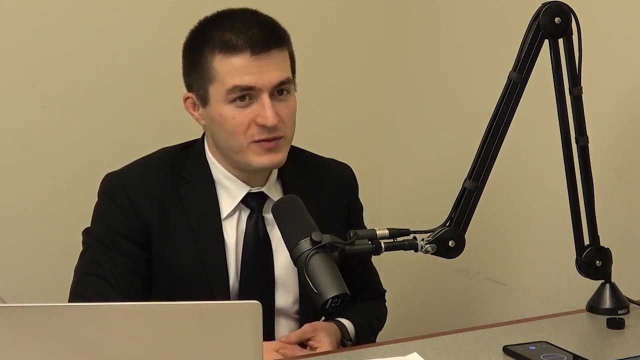 What is the best way to learn math for people who might be at the beginning of that journey? I think that's a question that a lot of folks kind of ask and think about. And it doesn't, even for folks who are not really at the beginning of their journey, like there might be actually deep in their career of some type, they're taking college or taking calculus and so on, but still want to sort of explore math. What would be your advice in sort of education at all ages? 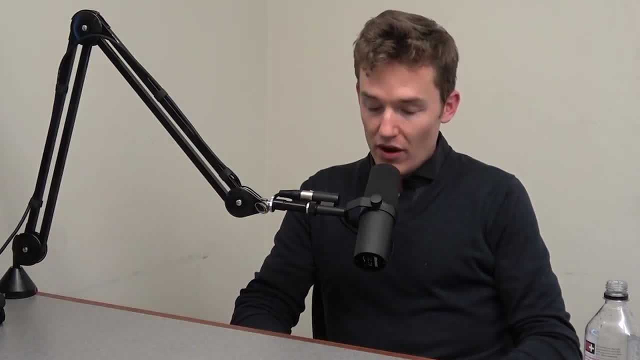 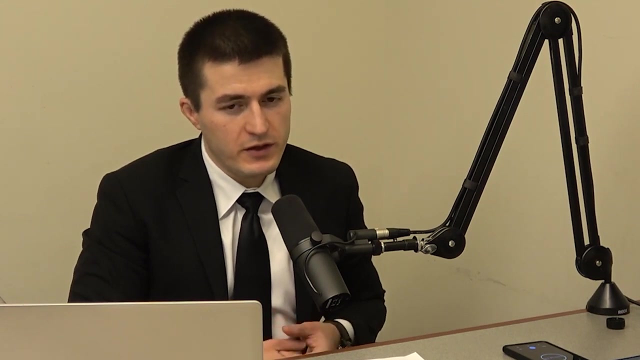 Your temptation will be to spend more time watching lectures or reading. Try to force yourself to do more problems than you naturally would. That's a big one. The focus time that you're spending should be on solving specific problems and seek entities that have well-curated lists of problems. So go into like a textbook almost and the problems in the back of a textbook kind of thing, back of a chapter. So if you can, take a little look through those questions at the end of the chapter before you read the chapter. 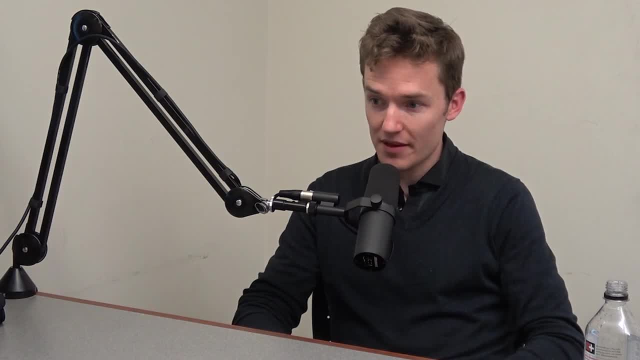 A lot of them won't make sense. Some of them might, and those are the best ones to think about. A lot of them won't, but just take a quick look and then read a little bit of the chapter and 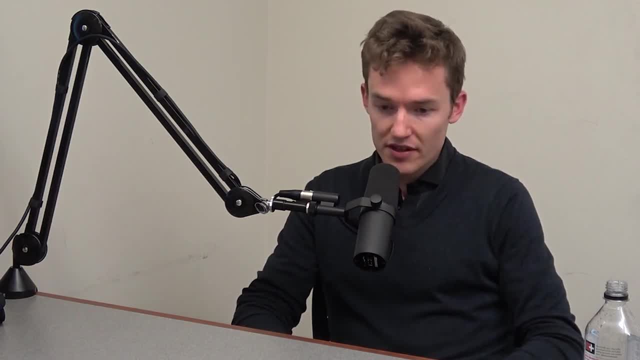 then maybe take a look again and things like that. And don't consider yourself done with the chapter until you've actually worked through a couple exercises. And this is so hypocritical, right? Because I put out videos that pretty much never have associated exercises. I just view myself as a different part of the ecosystem, which means I'm kind of admitting that you're not really learning. 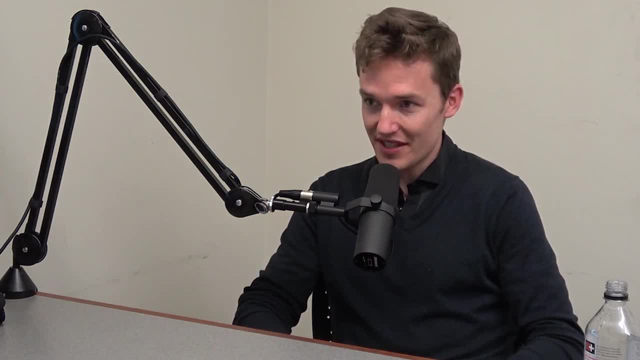 Or at least this is only a partial part of the learning process if you're watching these videos. 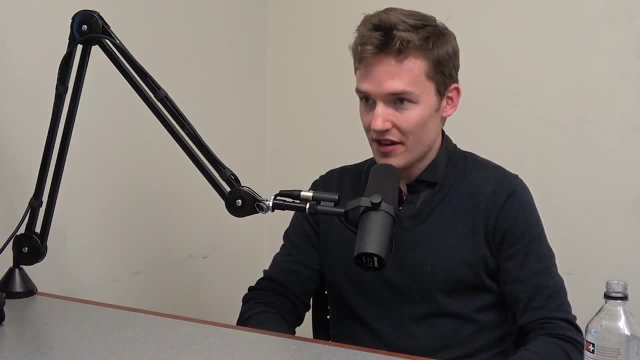 I think if someone's at the very beginning, like I do think Khan Academy does a good job. They have a pretty large set of questions you can work through. 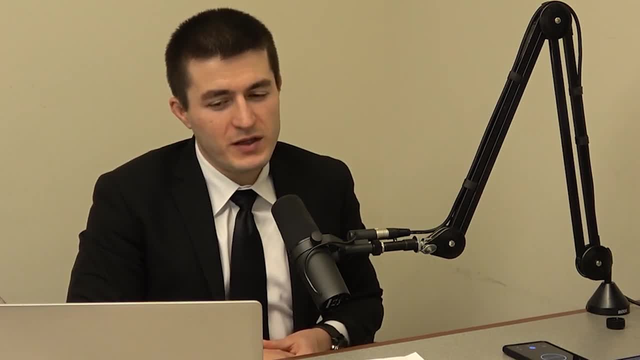 Just the very basics. Sort of just picking up, getting comfortable with the very basics of linear algebra or calculus on Khan Academy. 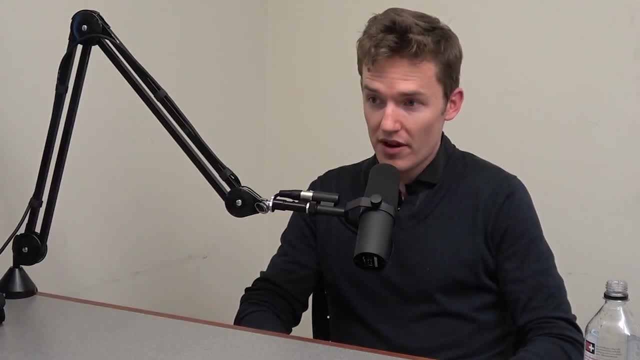 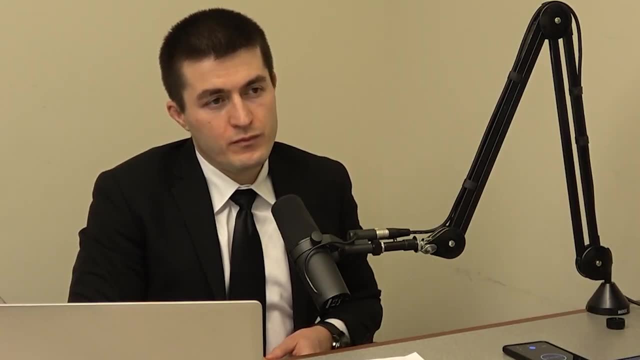 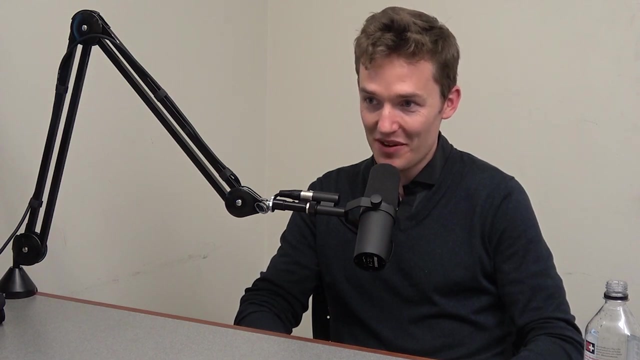 Programming is actually, I think, a great, like learn to program and like let the way that math is motivated from that angle push you through. I know a lot of people, I know a lot of people who didn't like math got into programming in some way and that's what turned them on to math. Maybe I'm biased because like I live in the Bay Area, so I'm more likely to run into someone who has that